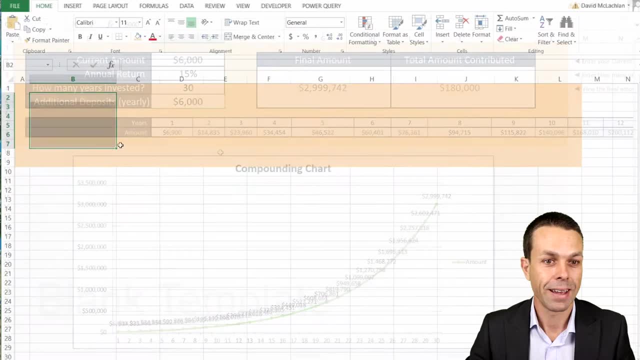 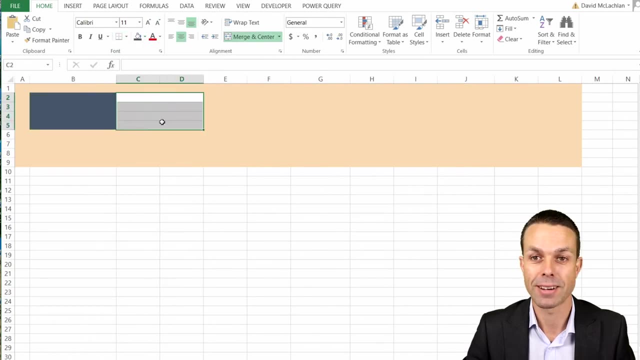 we're going to create in Excel. Let's get into the sheet Now. there are a few really neat little tricks that we're going to use while we're creating this sheet, But first, of course, we're just going to just create the general background. 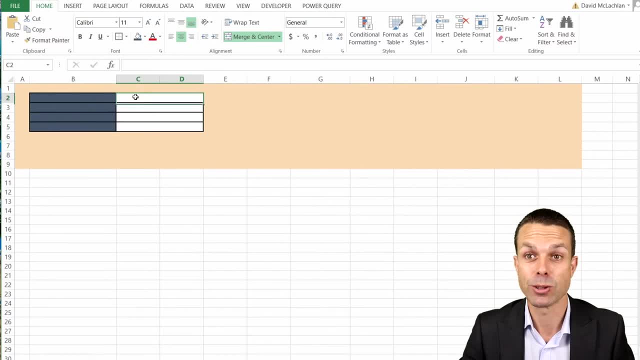 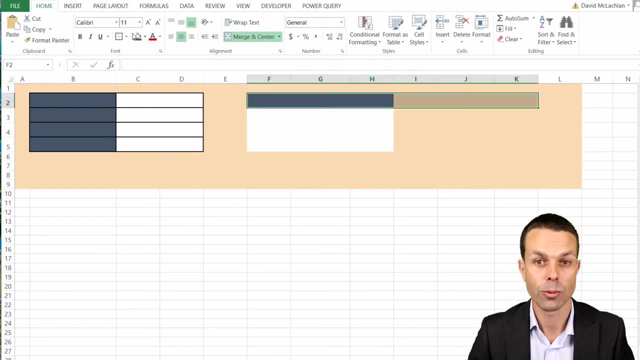 of our sheet And we can speed this up as we go along so that we can get into the real goods in a second. We just want to merge and center these particular cells. This one will be a nice deep blue. We'll just merge and center these particular ones, make them a. 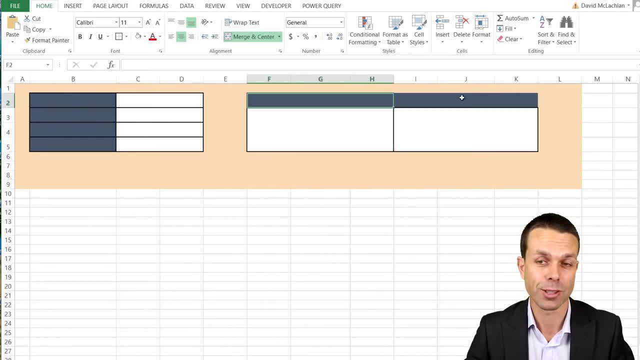 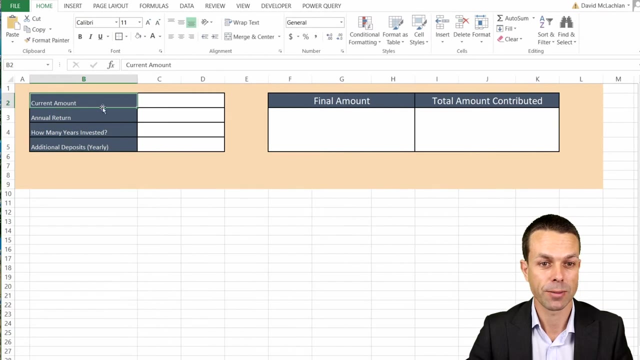 little bit bigger, And these are our final amounts and total contributed, So we can see how much we've contributed Over time. and, of course, a thick border around all of these as well. We'll make these ones over to the right and just increase the indent a little bit. Now that's looking really quite. 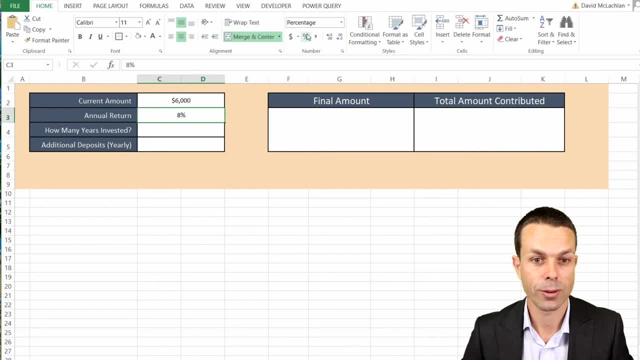 nice. This is where we might put our current amount. for example, Our annual return might be 0.8,. but we'll turn that into a percentage And there we go. That's a little bit better. We can give that some decimals if we really want to. 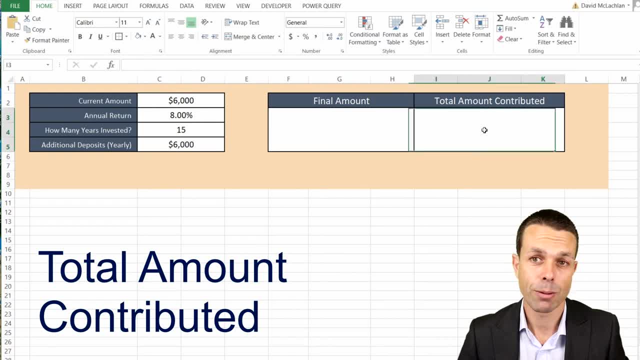 How many years will we invest it for? Maybe we'll put any number there. Now we want to figure out the total amount that we will contribute over time And we can just put that in the center here. So to get our total amount contributed, we want to say this is going to be equals and it'll be all of. 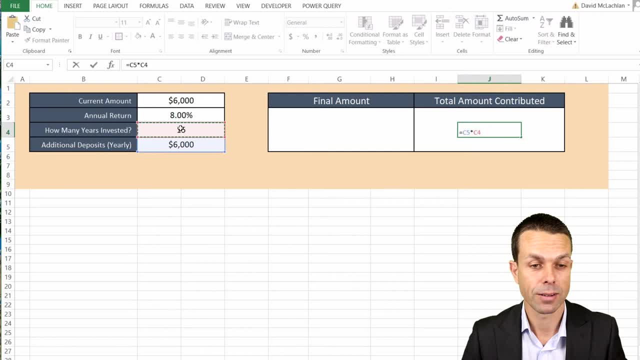 our deposits multiplied by the amount of years that we're doing it for. so 15 years. But we also want to add the initial amount at the very beginning. So if we do all of that, then that gives us our total amount contributed. And we can see that we've contributed a little bit more. So we can see that we've contributed a little bit more. And we can see that we've contributed a little bit more, And we can see that we've contributed a little bit more. So that's that. 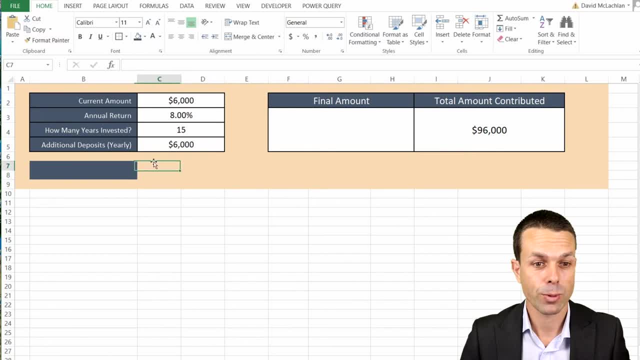 And that's really good. That's a great start. Now let's look at the final amount. But to do that, first we're going to have to create the compounding table, And this is where we're going to be able to get all of our data from. 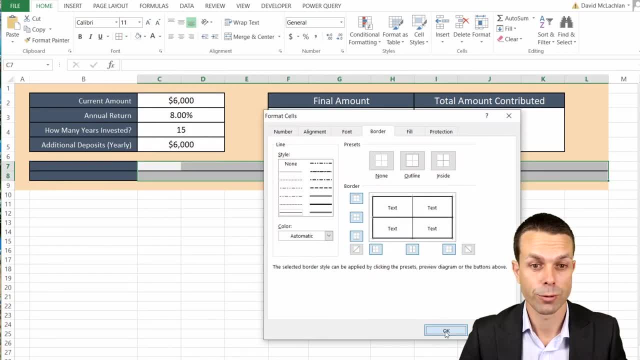 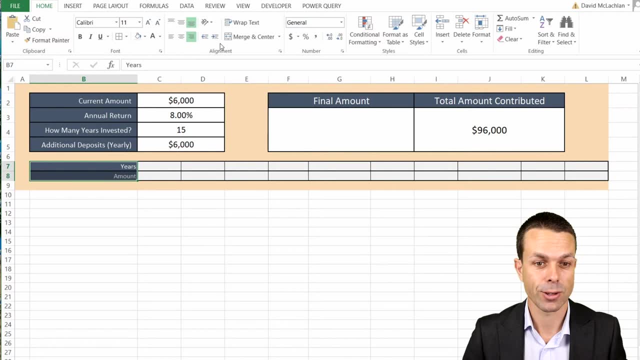 And so this is going to be really important. Just do a few more borders here, And we'll give ourselves a nice normal border in between And increase the indent ever so slightly. Now, these are the years that we're going to be investing for. So, all the way up And for, 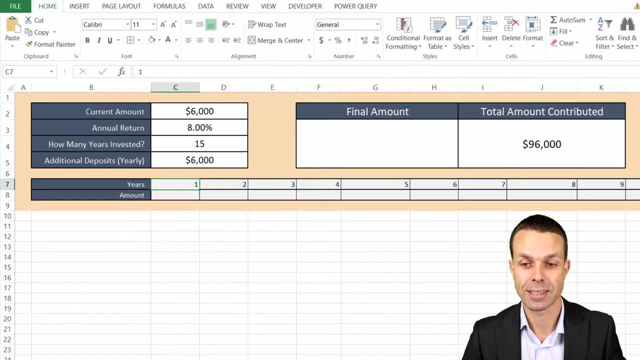 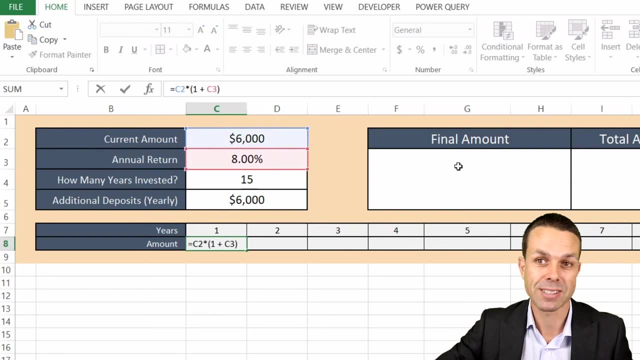 the rest of these we can just increase And let's see, let Excel do the work there. We'll center those, But for the amount- and this has to increase over time- and use the reinvested returns as well. so it gets a little bit tricky, But what we're wanting. 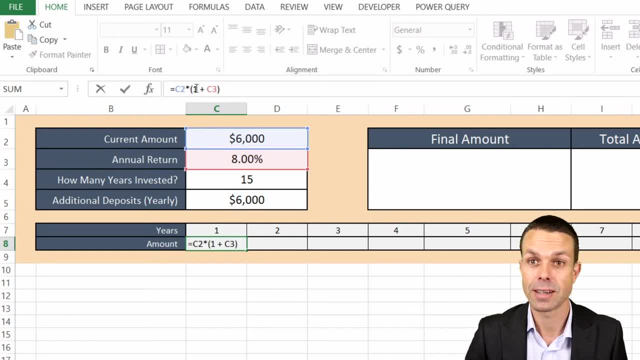 to do is have our current amount, which is 6,000 currently, multiplied by 1 plus 8%, so 1.08, basically, is what we're having, And so that's our first amount, But the second one's going to be a. 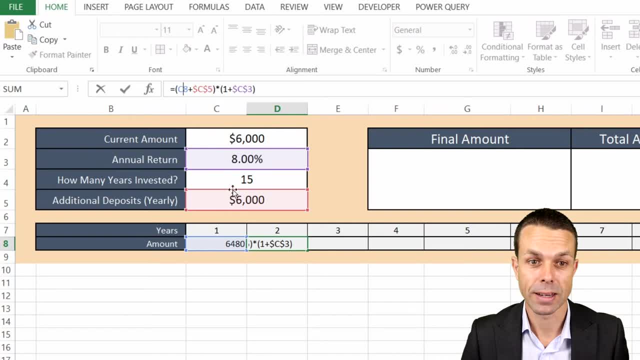 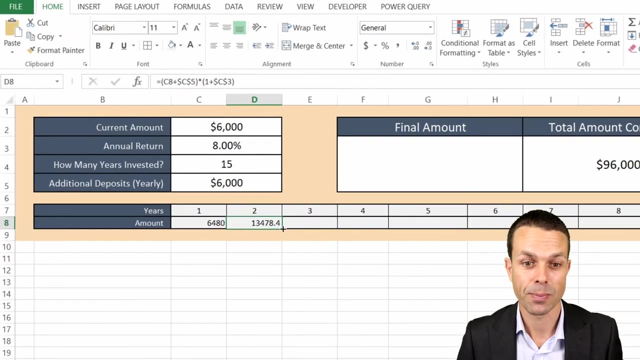 little bit different. And the second one is going to take our previous amount here and add the additional yearly deposit and then multiply that by our 1 plus 8% as well, so 1.08 as well. So once we do that, that gives us our total amount plus the contributed amount, and that's how the 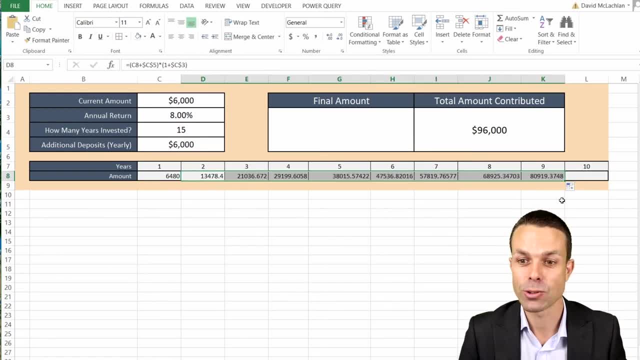 snowball starts to begin If we drag this all the way across and we'll just reduce the decimals ever so slightly. Now we've got up to 10 years of our compounding amount based on the information that we've put in here. Now it's really important to 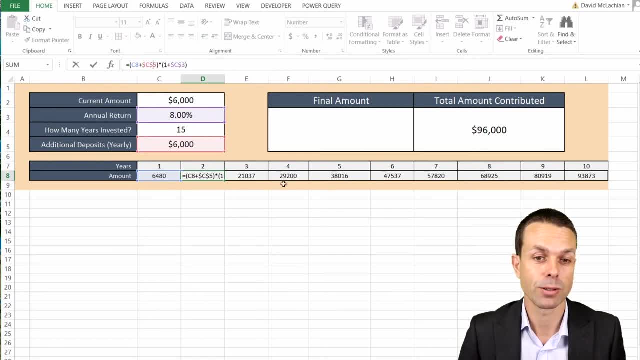 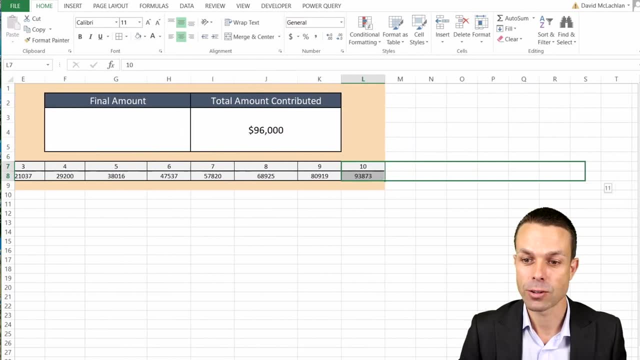 put a dollar sign in front of the C for these ones, because we don't want that to move when we're dragging that across. So that's really, really important. But now that we've done that, we can just take this and keep dragging this across and hopefully this will keep going. So we've got 11,. 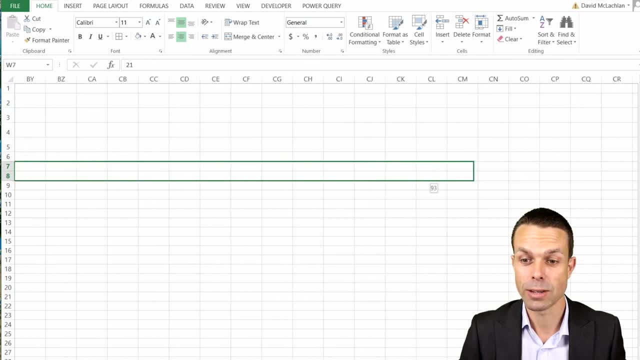 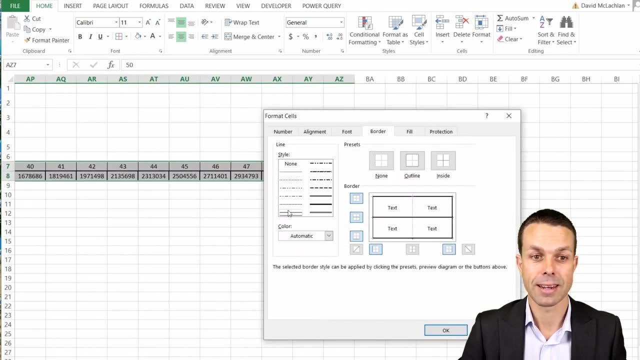 12, and all the way. Now it's really starting to increase. We can even keep going up to 30 or 50 years if we really want to, And if we've got our 50 years, we might just select that again and do. 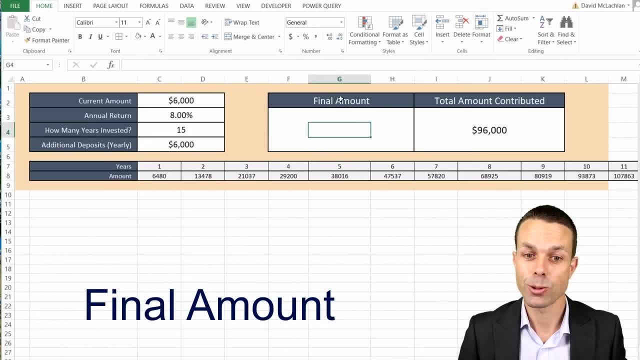 our borders and make it a little bit nicer. We can use this to figure out the final amount, based on this little table that we've created for our compounding amounts. So let's see what we've got For our final amount. we're going to use index and. 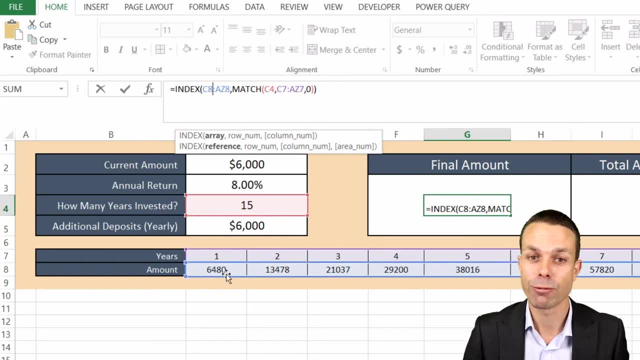 match And the index function. once we do that, what we're looking for first is the amount row that we've just created, So that nice amount row all the way down there up until however long we want that to go for. But then, when we get to the row number that we want to index that against, we want. 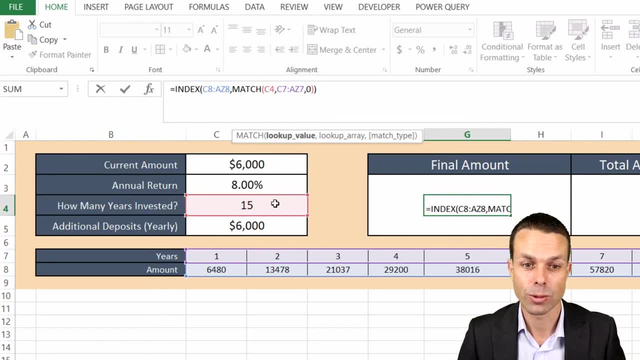 to match how many years invested, So C4, which in this case is going to be 15 years, but it could be anything- And then we want to match that to look up against the years row that we've got up the top here. So using index and matching that to the years invested and the years row here, if we select. 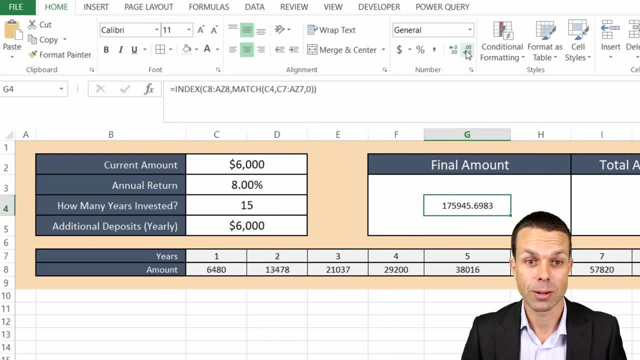 enter. now that gives us a final amount And we'll just tidy that up ever so slightly and reduce the decimals there. Now we've got our final amount based on all of the data. So we've got our final amount that we've put in, But we still want to create a chart and make sure that that looks really nice. so 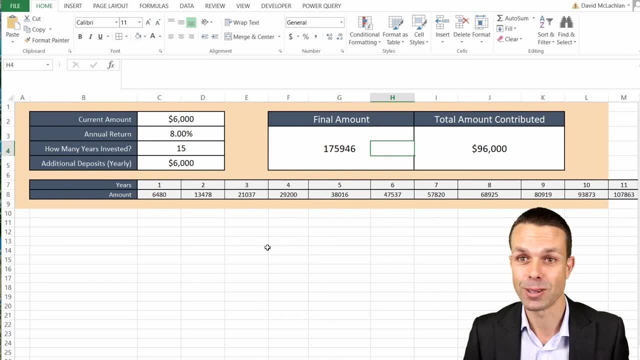 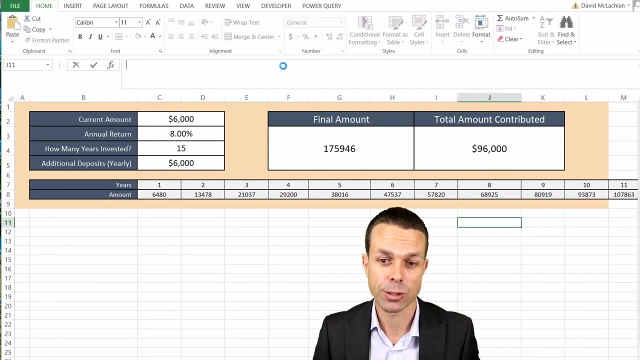 we can visualize how long it takes us to get to a million dollars if we need to. And to create that chart we need that to update dynamically. So we're going to create a named range, But to do that we're also going to use a formula called offset, And so that's going to offset against these numbers. 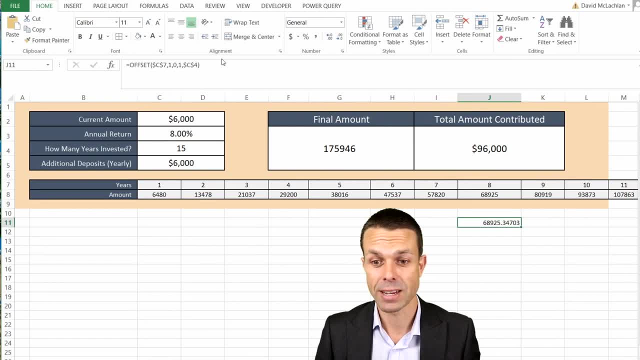 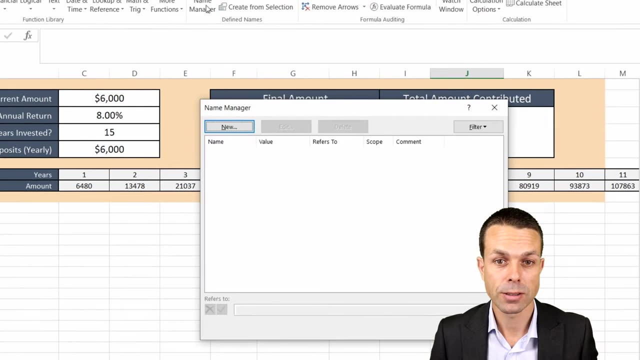 on our chart when we need it to, And so for that to update dynamically. So that's the formula there, So we're going to put currently, But what we really want that to do is we want that to be used in our named range. So let's create that. We go to formulas and we go to name manager. Now we want a new name. 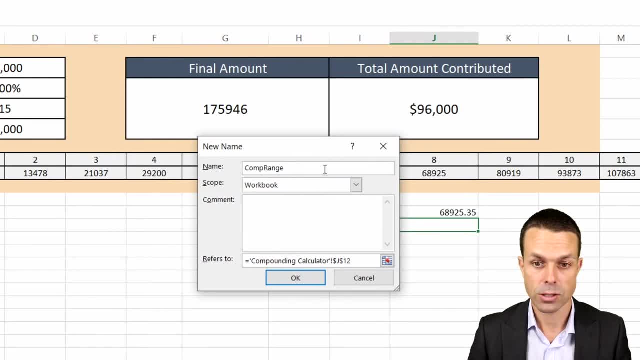 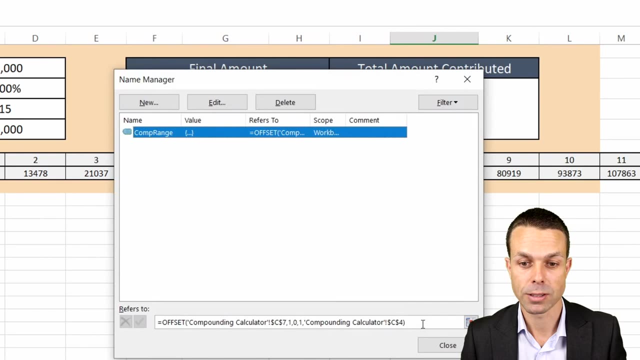 And let's say: this is our compounding range, or comp range, You can name this anything you like, of course, And we want this to refer to an actual formula. So we're going to say we're going to put in that formula that we had before, which is offsetting against the numbers, And we'll just 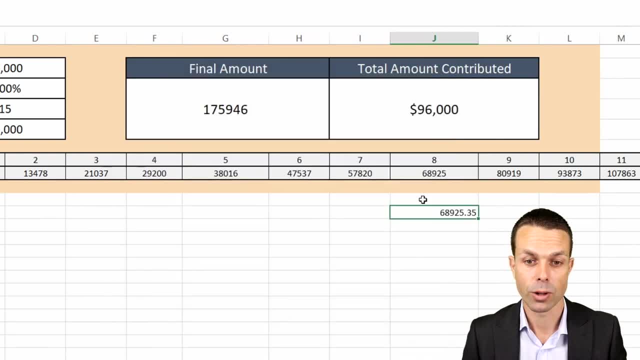 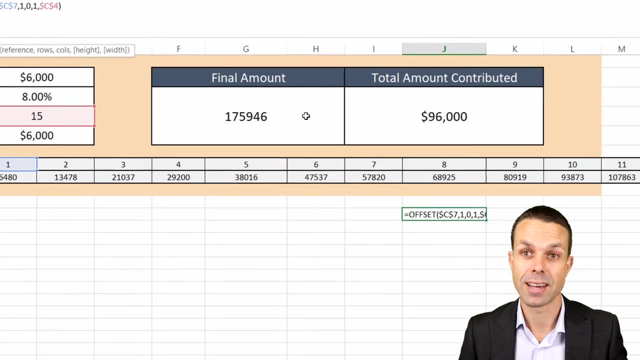 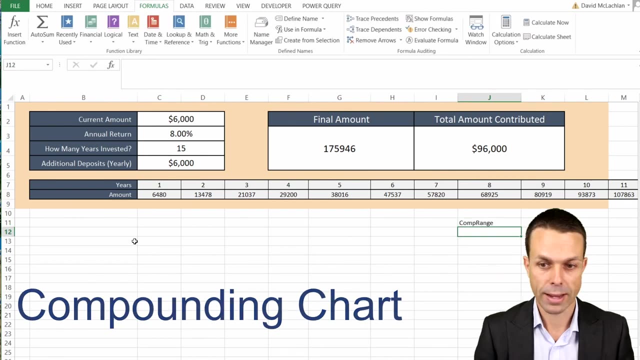 click enter there so we can see what it does. We'll close that off. But, as you can see, it offsets against the numbers, So the how many years invested, And it does that against our years row, just like we set up for our final amount Now that we've got our named range of comp range. 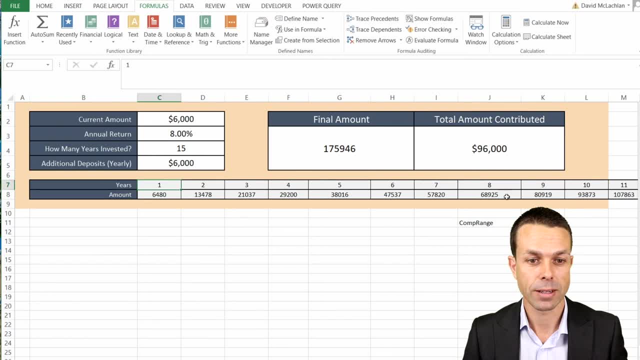 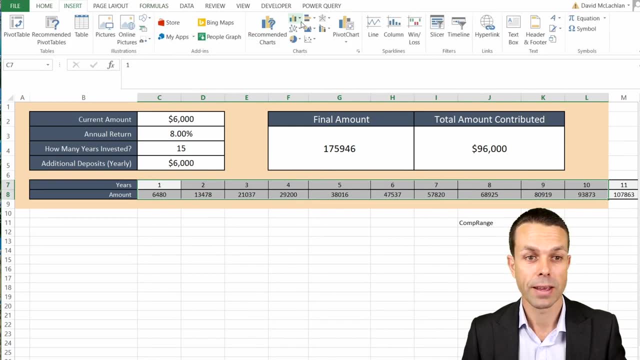 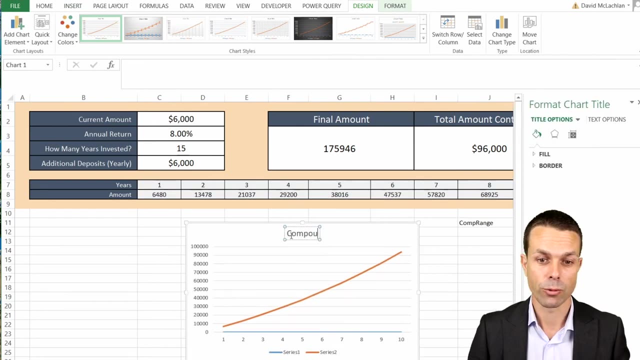 all we need to do is let's select our amount here. In fact, we can select some of anything in this particular compounding chart or table here And if we say insert and we'll insert a line chart, Now we've got our normal line chart. We can rename this to. 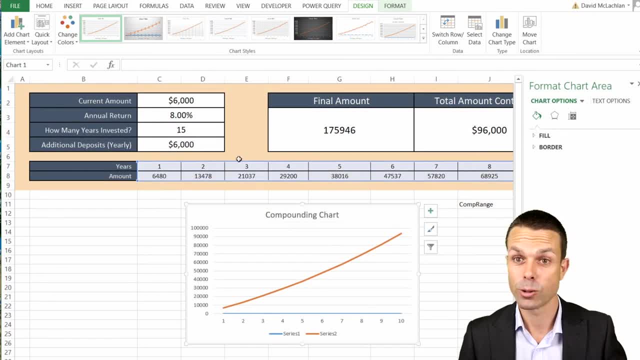 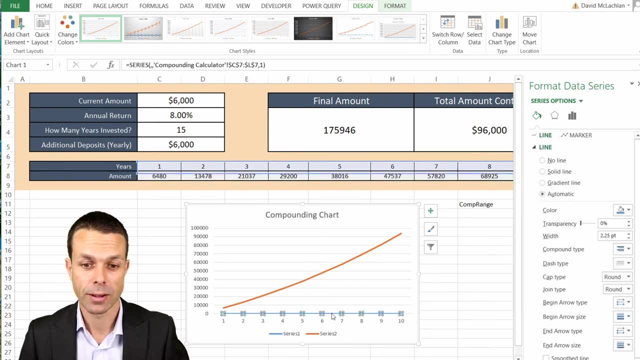 compounding And, as you can see, it is already doing a good job of creating a nice compounding chart, But we still want it to update dynamically, based on the information that we select over here. So we'll just get rid of that second series. Now we've got a beautiful line, But what we want to do 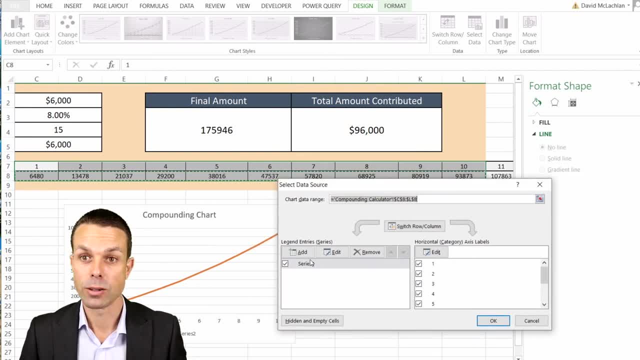 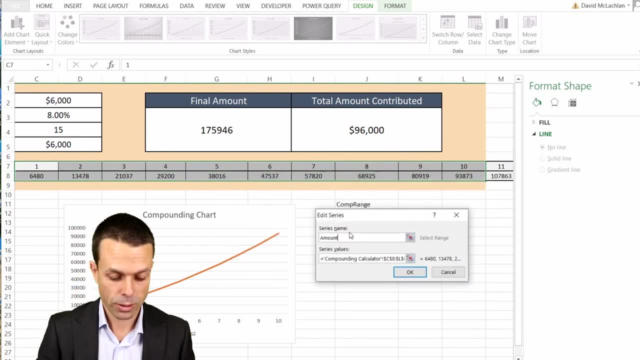 is right click and select data, And what we're going to do is just edit the series that we're using for this particular chart, And we're going to do that, And we're going to do that, And we're going to call it amount. We'll call it the amount And with the amount we've got our compounding. 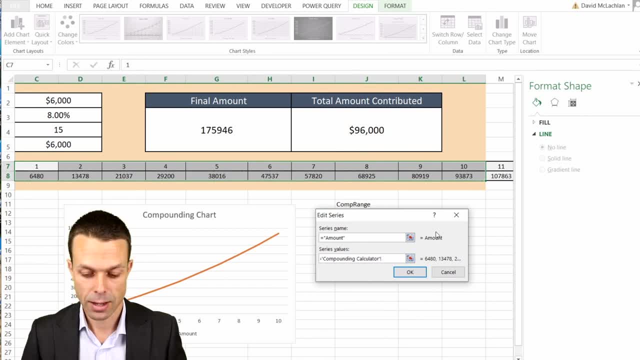 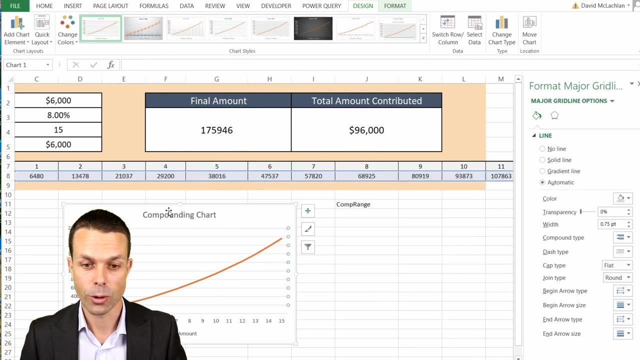 calculator sheet And we just want to get rid of the reference there And we want to turn that into the comp range instead. So that's the named range that we just created And let's see if we select enter there And that does seem to work And so if we click OK, now all of a sudden this does give. 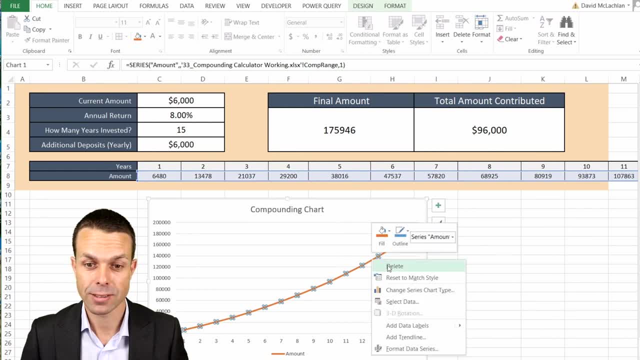 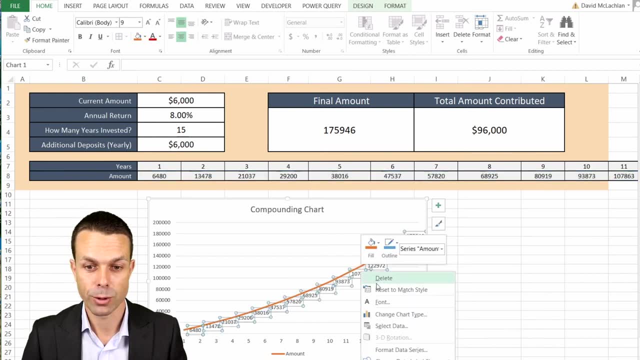 the information that we're looking for, the final amount, As you can see, it's around the same area. If we add data labels, let's see what we've got here. Oh, there we go. That's very beautiful We. 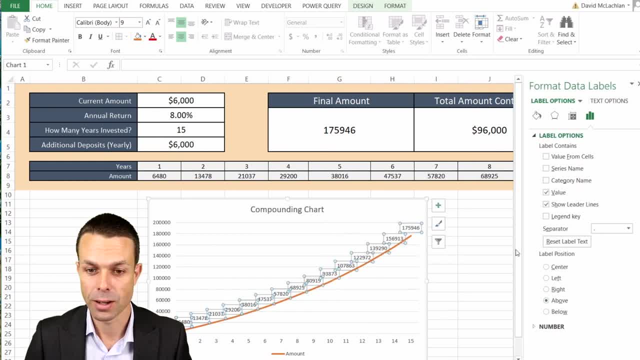 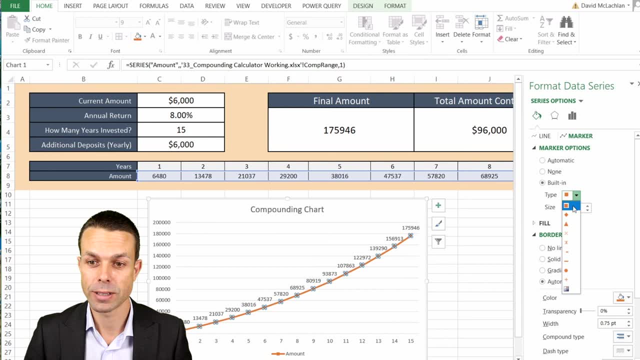 can format those And we can put them on the top or on the bottom, wherever you prefer. And let's say we want to add some markers here. If we select our line and we'll just go to marker over here- marker options, We want some marker options. Maybe we'll select a nice round one there. 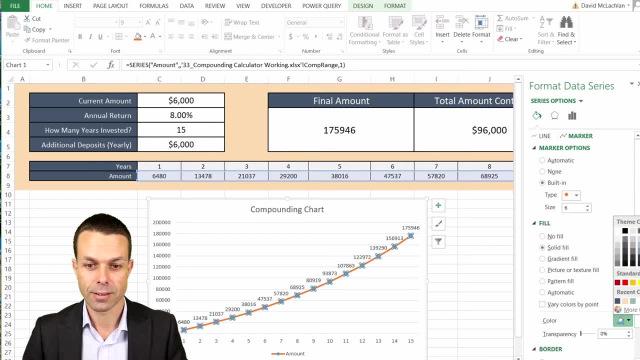 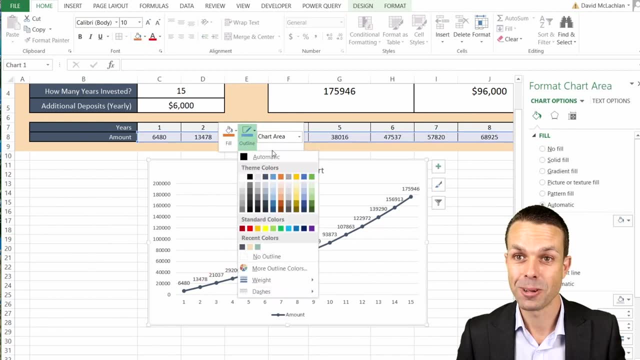 make it a little bit bigger if we want. And yeah, now we can see, maybe we can change the color here and change the color of our line if we really want to as well, Now we can really see that this chart has updated dynamically for us And 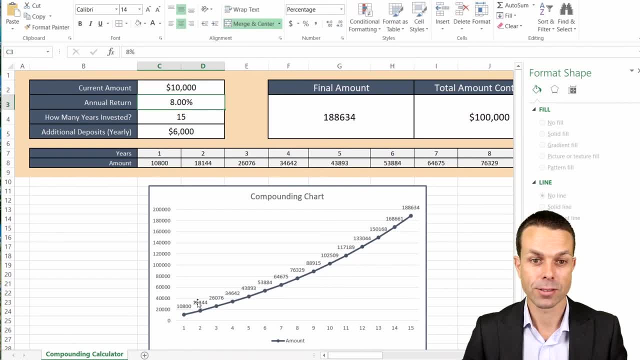 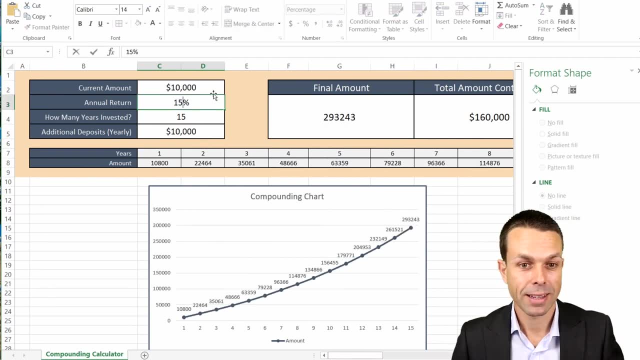 let's try and let's say we want to start with $10,000, for example: OK, now it's updated that as well. Let's say we put $10,000 in every year And let's say we managed to get 15% annual return. 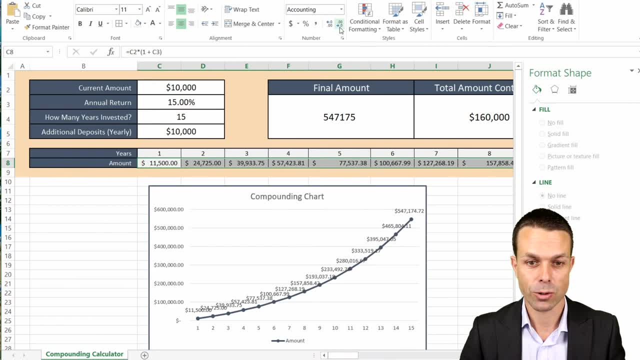 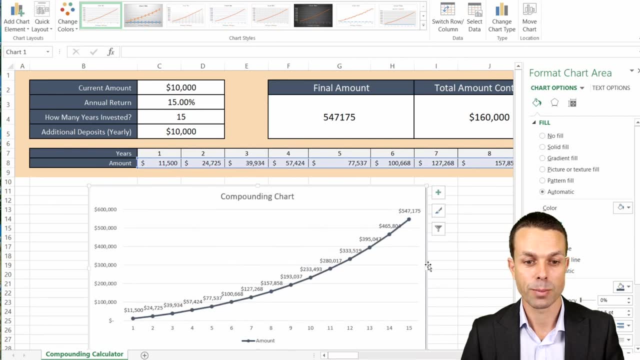 Oh, the data of course doesn't have any dollar signs, So let's just quickly select all of those and give ourselves some dollar signs. There we go. That's a little bit better, And we'll just make our chart a little bit bigger so that it can fit all of.